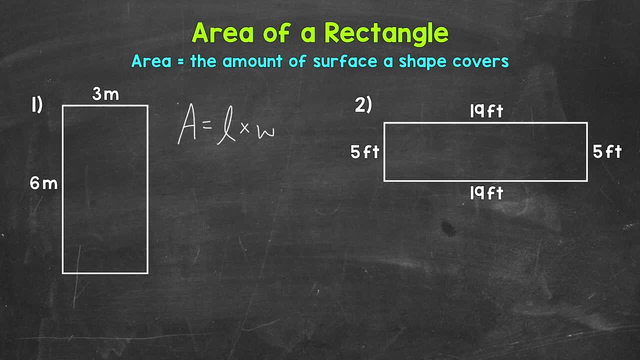 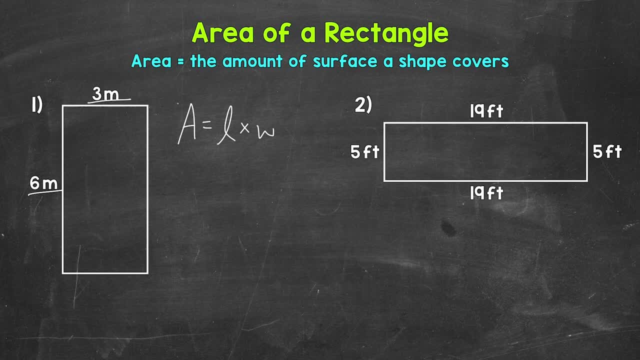 the longer side for the length. So I'm going to use the longer side for the length. So I'm going to use the longer side for the length. So I'm going to use the longer side for the length, So six meters, and then three meters for the width, So area equals six meters times three meters, And 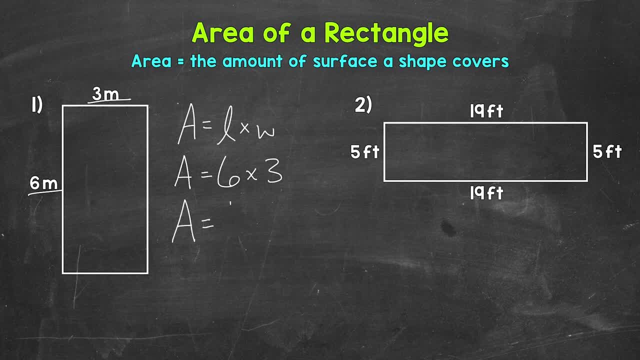 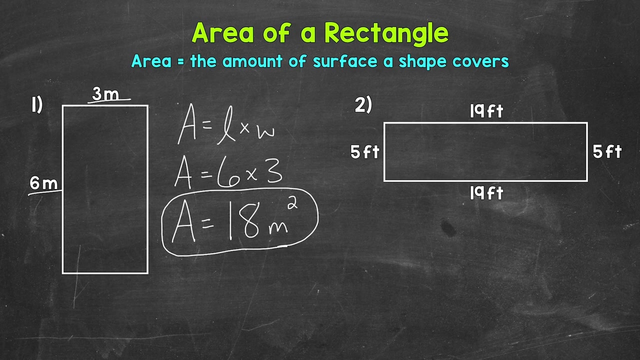 now we can multiply Six times three gives us an area of 18 square meters. We measure area in square units, so this is square meters. Before we move on to number two, let's take a look at why we do length times width and look at a visual of area. we have six meters by three meters, so let's draw these. 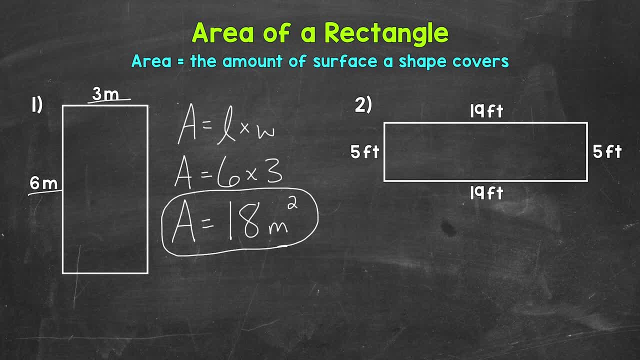 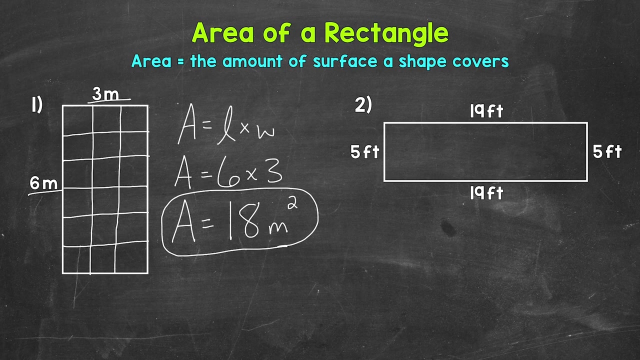 out, starting with six meters. so i'm going to mark each meter here. so one, two, three, four, five and six. so we have six meters there and now we can do the width. so three meters, one, two and three. you'll notice that we have squares now. these are square units and 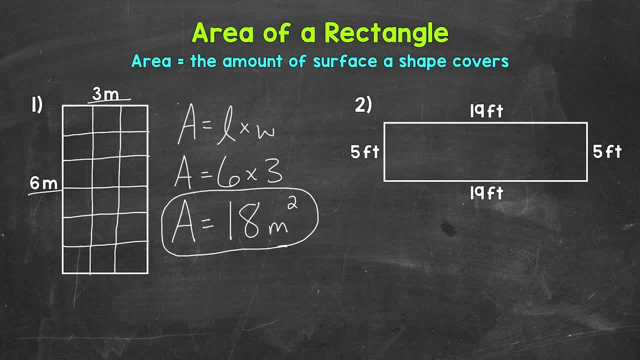 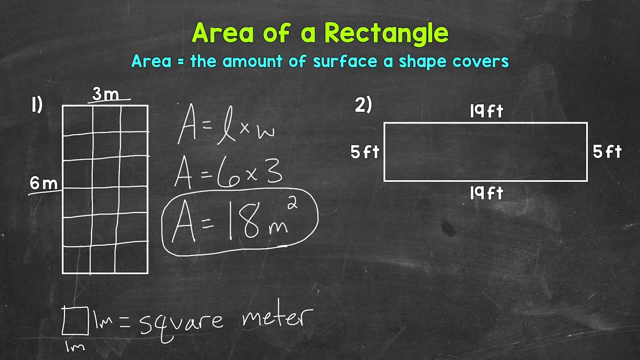 specifically for number one, those are square meters. that just means that each square is one meter by one meter, and this is a square meter. when we find area, we find how many square units something covers. so for number one, how many square meters does this rectangle cover? well, one, two, three, four, five, six, seven, eight, nine, ten, eleven. 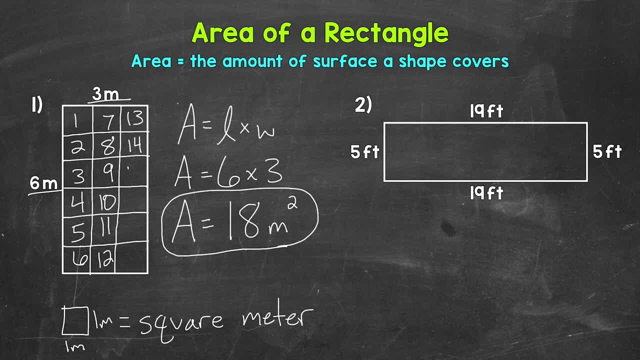 twelve, thirteen, fourteen, fifteen, sixteen, seventeen, eighteen, which is exactly the same thing we got by doing length times width. so by drawing all of that out, this helps us visualize area and square units, but it's much quicker just to do length times width. let's move on to number two, and for this one we're just: 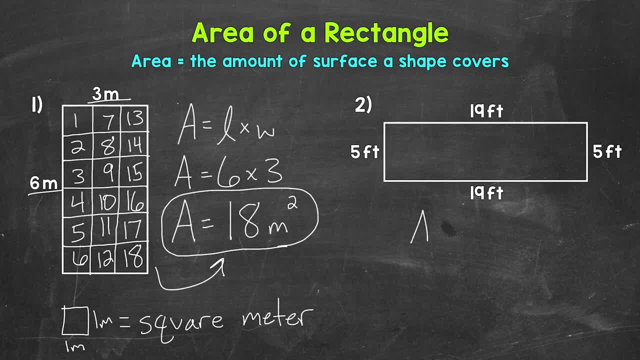 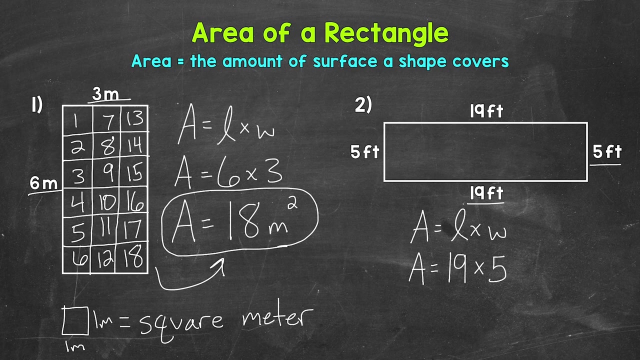 going to use the formula. so area equals length times width. so let's plug in the length. we're going to use 19 feet, so 19 feet times the width of five feet. so again, i used the longer side for the length. now for number two. it's a little. 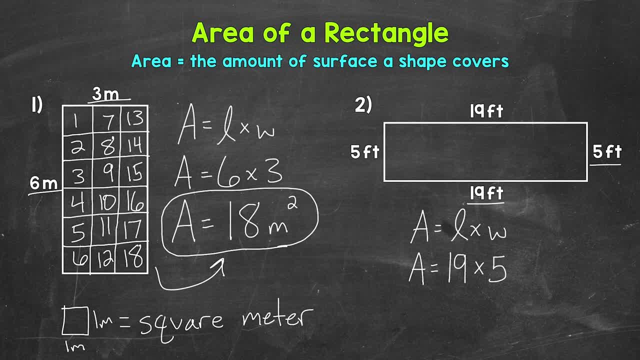 different than number one because all four side lengths are written out. that doesn't mean we need all four side lengths. we least need the length for sorrow long side length number two. it would be going to be down on all of the side lengths. that's going to be in the inner right corner, so we'll get. that first point, because we need all the hundred feet in length. so really you didn't get all fourty, and then we got ourselves over with your own pie. we came to my last point and i'll give you a little more time. just is this way: 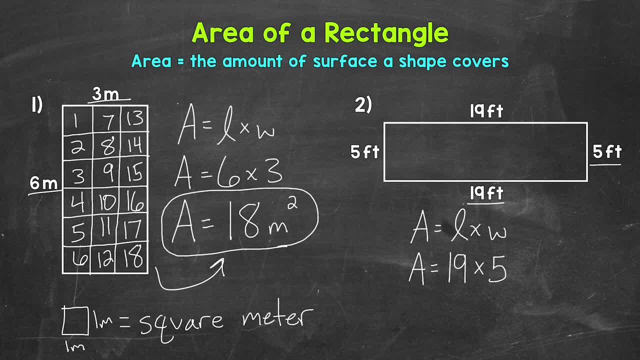 that both of your side recorded. 2 feet equals five feet, and then we're going to be drawing and× können. i'll try to divide them and then we're going to combine them. still just need the length and width. We're not multiplying everything. that's. 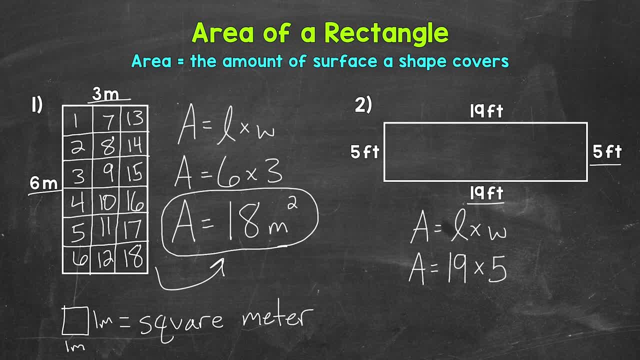 written out or given, so something to keep in mind. Now we can multiply so: 19 times 5 gives us an area of 95 square feet. So there's how to find the area of a rectangle. Let's move on to finding the. 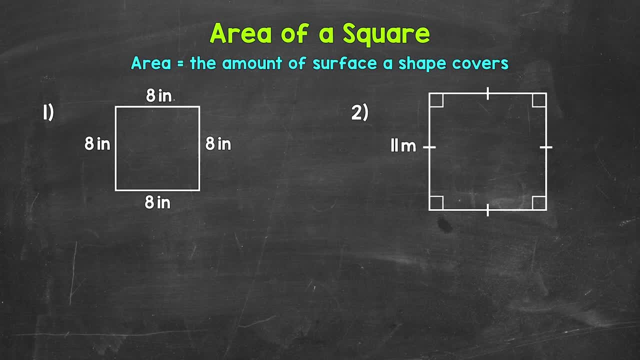 area of a square. Now we're going to take a look at how to find the area of a square. Let's jump into our examples, starting with number 1, where we need to find the area of that square. Now for squares. we can find the area by: 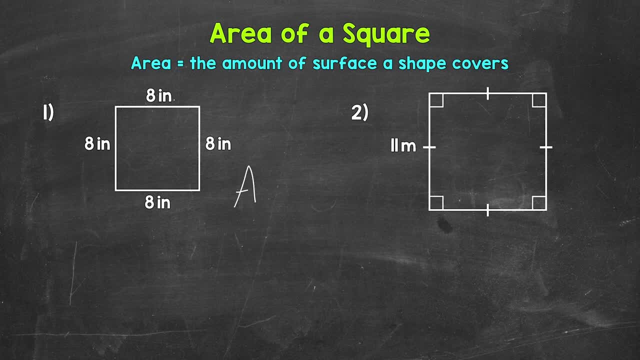 squaring a side length. So we can use the formula: area equals a side length squared And for this square, each side length equals the square area squared. foiI de gu Mil domina maili is 8 inches, So let's plug in 8 inches here for our side length. So 8 squared. 8 squared means 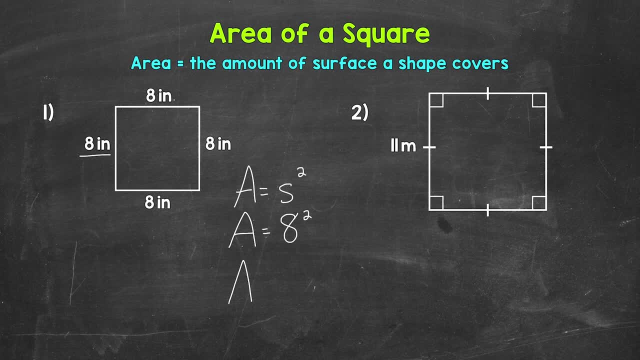 8 times 8, which gives us an area of 64 square inches. Let's move on to number two, where we have a square with sides that are 11 meters, And you'll notice that we only have one side labeled. That's because this is a square and we know.